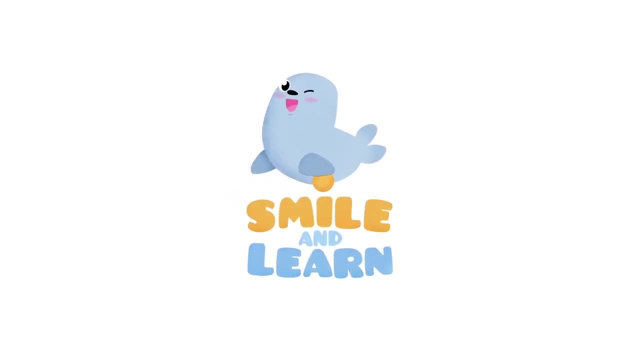 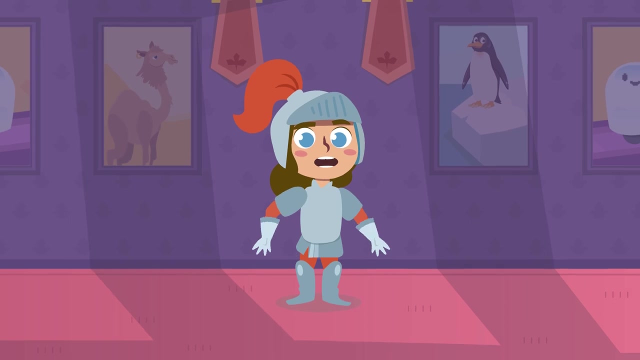 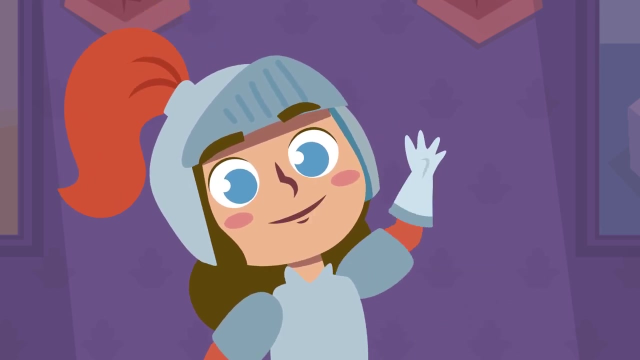 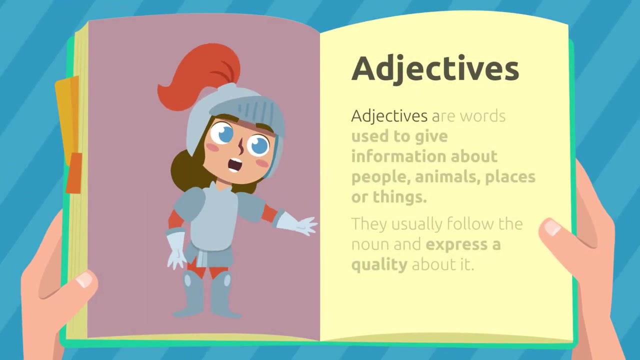 Smile and Learn Greetings, word-lover friends. Today we will continue learning more adjectives. What do you say? Do you remember what adjectives are? Don't worry, I'll help you. Adjectives are words used to give information about people, animals, places. 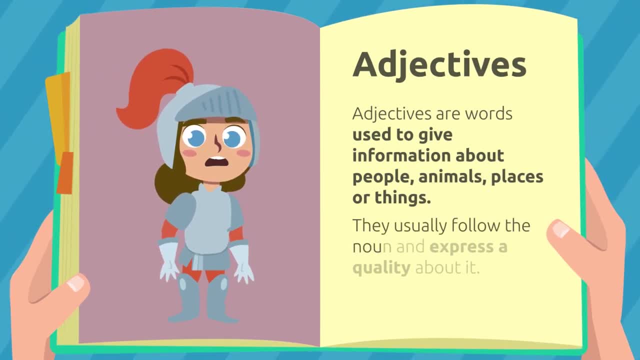 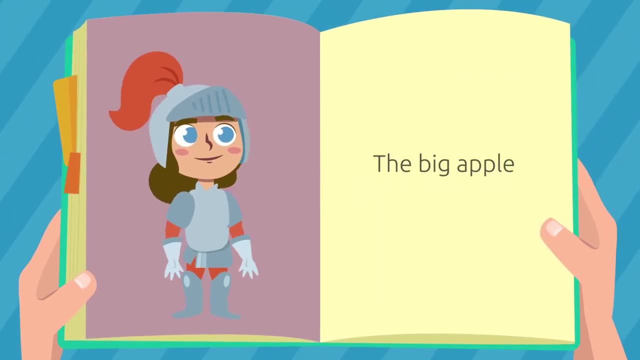 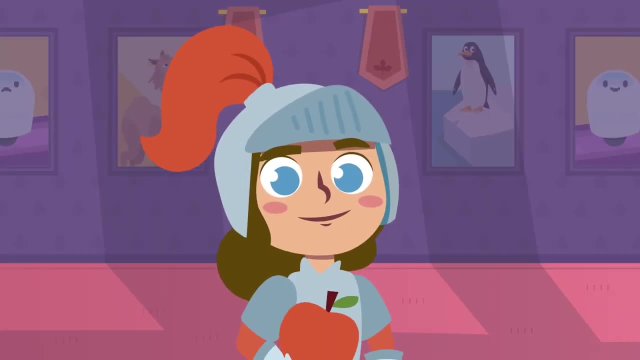 or things. They usually follow the noun and express a quality about it, For example, in the sentence the big apple. Big would be the adjective because it tells us what the apple is like. In this video, we're going to learn some adjectives that describe qualities about different objects. 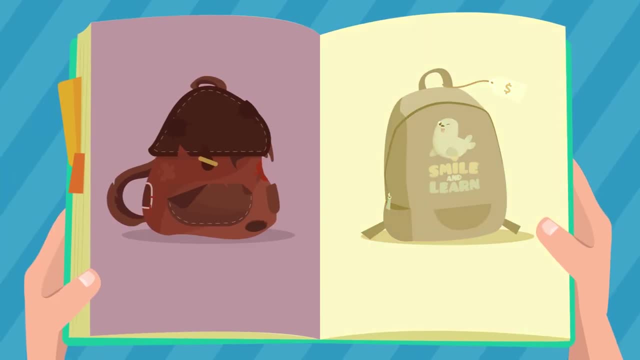 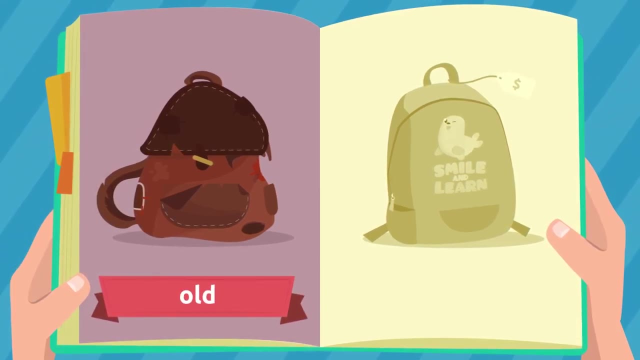 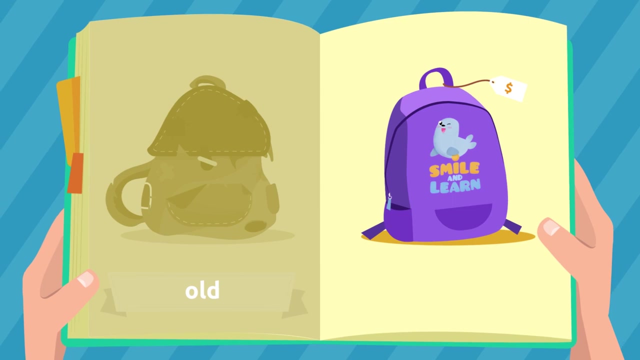 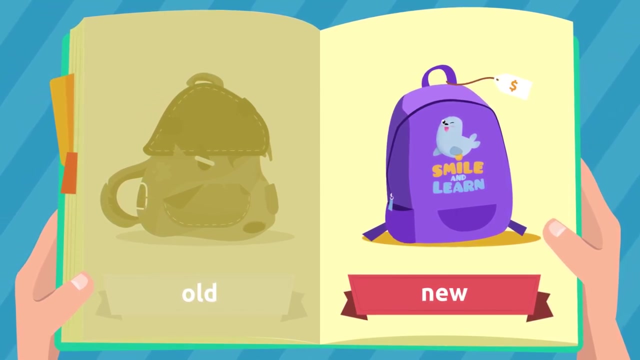 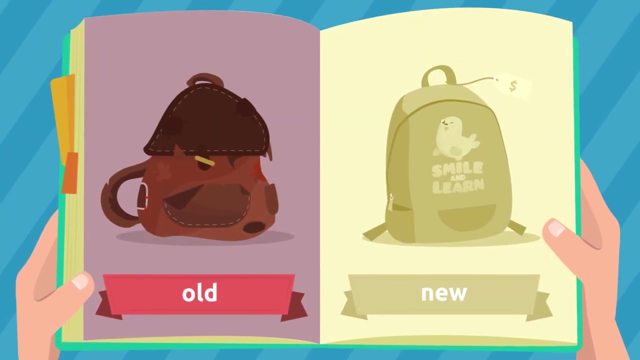 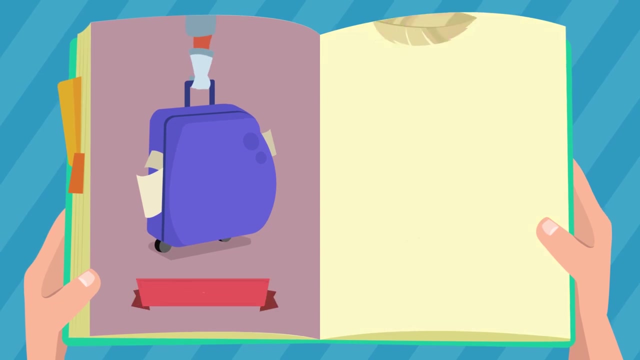 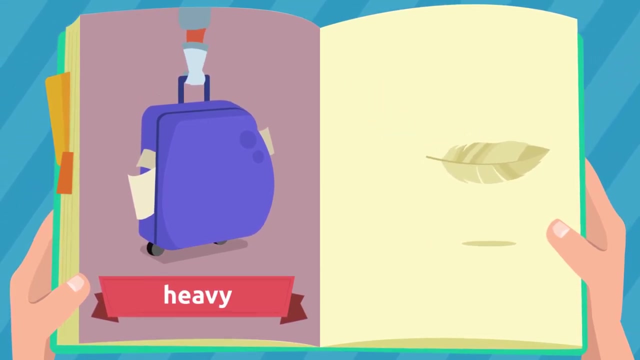 Let's begin. This backpack is old, Old, Repeat after me, Old. But this backpack is new, New, Repeat after me, New, New, Old, New, New. This suitcase is heavy, Heavy, Heavy, Repeat after me. 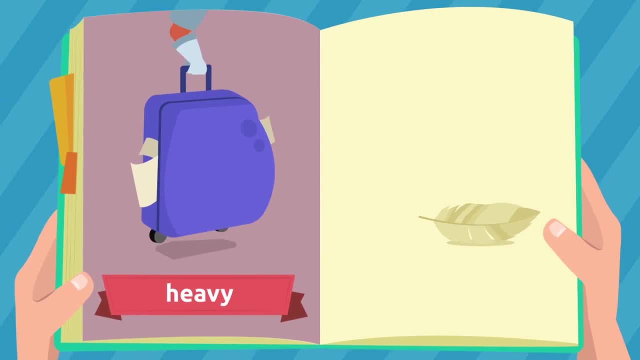 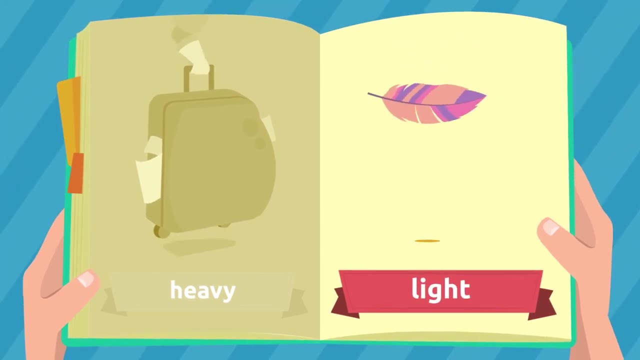 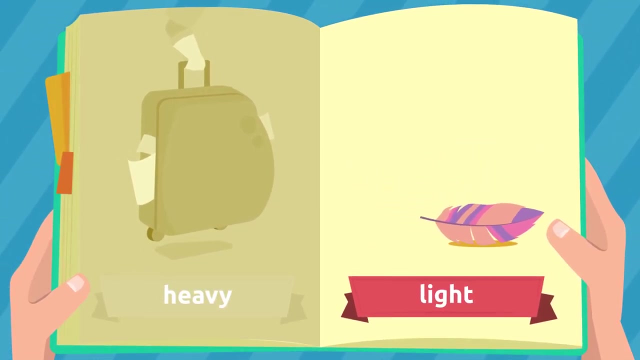 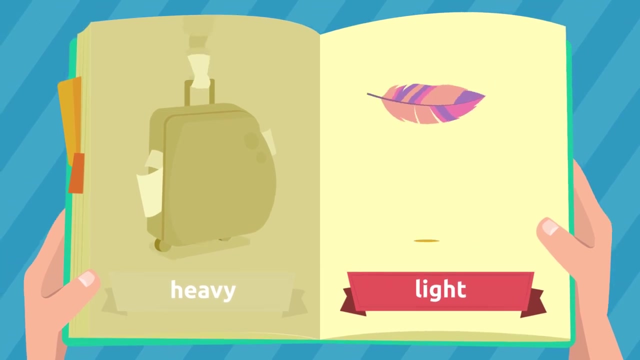 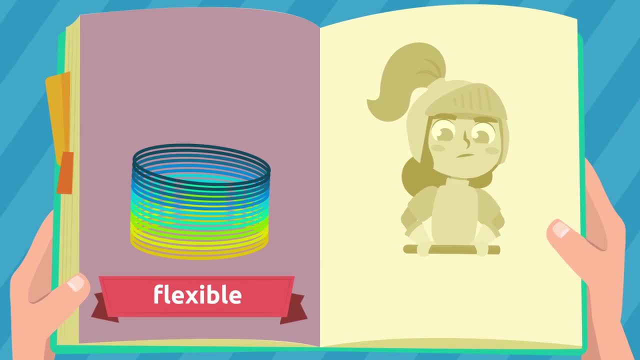 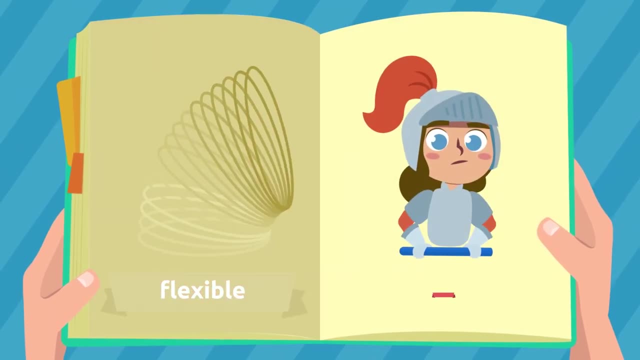 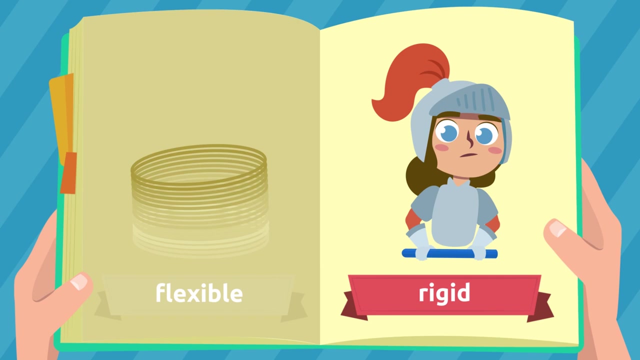 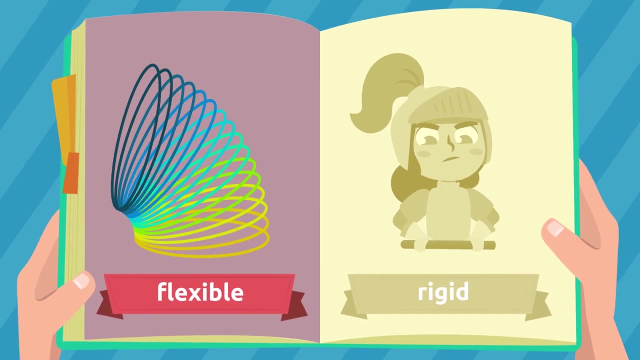 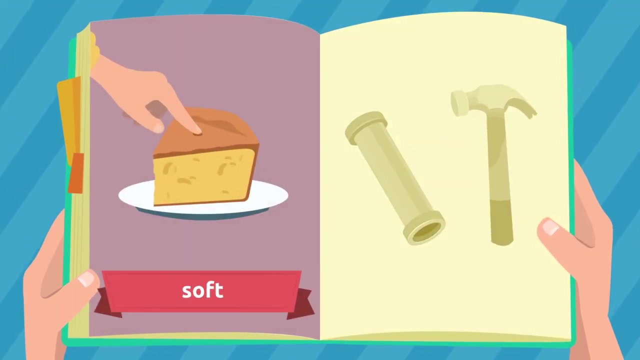